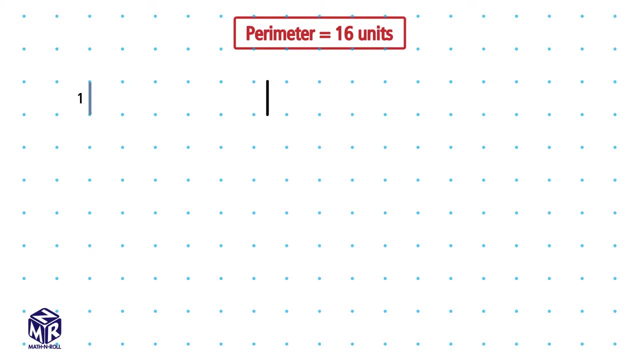 So if we choose one side to be 1 unit, the opposite side will also have 1 unit. We need to find the length of the second pair of sides of this rectangle. To do this, we subtract the sum of the two sides- 1 plus 1 equals 2, from the perimeter, and we get 14 units. 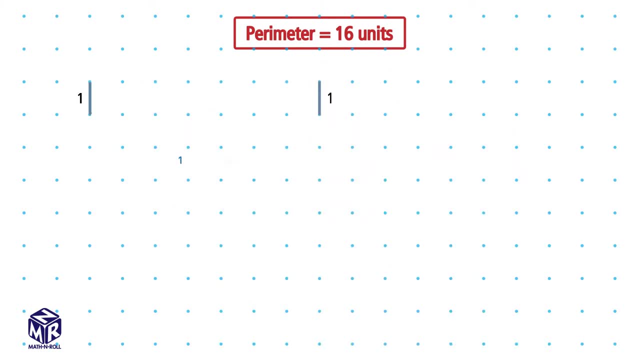 We have a pair of sides, so we need to divide 14 by 2 to get 7.. So now we know that this rectangle with a perimeter of 16 has two 1 unit sides and two 7 unit sides, Let's draw. 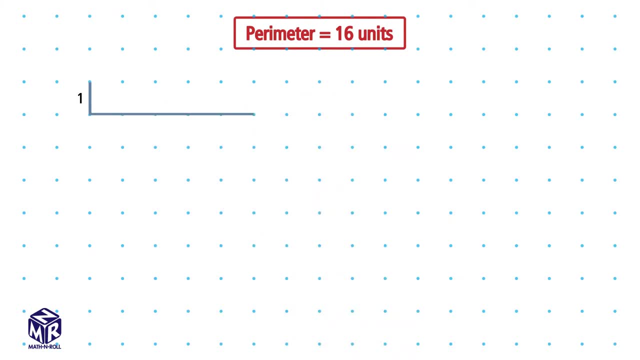 it out: We draw 7 units on the horizontal side. We go 1 unit up and then 7 units left. Rectangle A has a perimeter of 16 units and an area of 7 square units. Now let's draw another rectangle with a perimeter of 16 units, but this time let's make the shortest side. 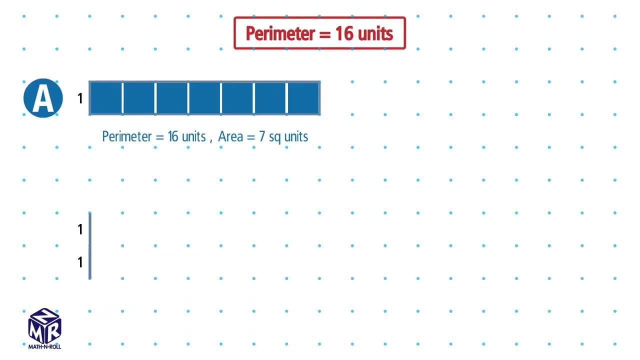 equal to 2 units. The opposite sides of the rectangle are both equal. To find the length of the horizontal sides, we have to subtract the sum of the two sides: 1 plus 1 equals 3.. We need to find the length of the horizontal sides: 1 plus 2 equals 3.. So now we have 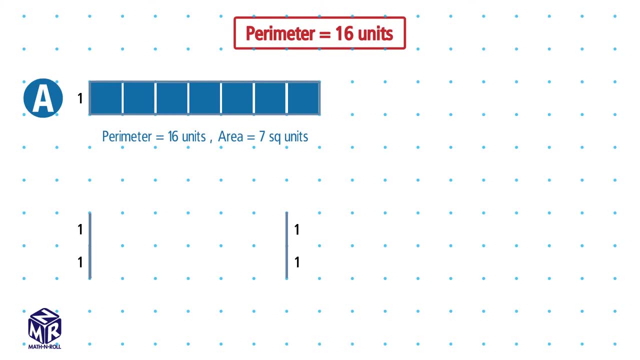 a pair of sides and we need to divide 12 by 2 to get 6.. The sum of the two sides is 4.. We subtract 4 from 16 to get 12.. We have a pair of sides, so we need to divide 12. 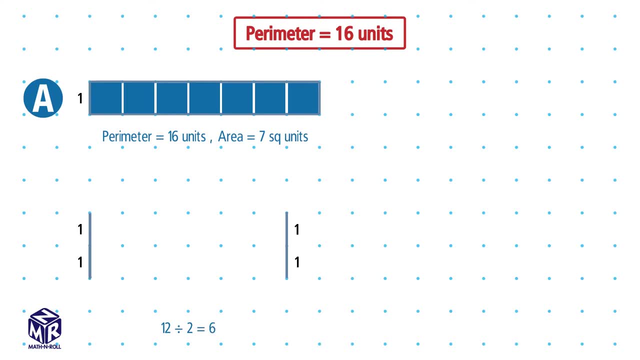 by 2 to get 6.. Now we know that this rectangle has a perimeter of 16, with two 2 unit sides and two 6 unit sides. Let's draw it out. We draw 6 units for the horizontal side, We side go 2 units up and then 6 units to the left. 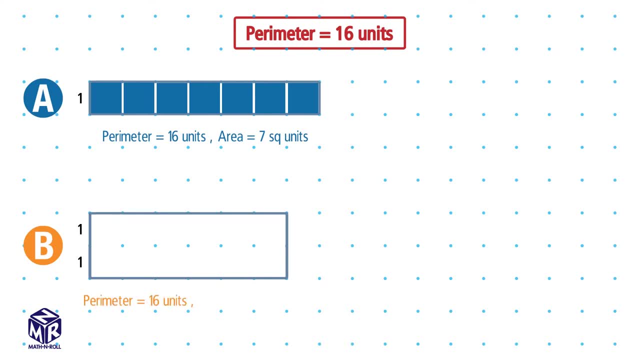 So rectangle B has a perimeter of 16 units and an area of 12 square units. As you can see, rectangle A and B have the same perimeter but different areas. Now let's draw another rectangle, but this time the shortest side will have 3 units.